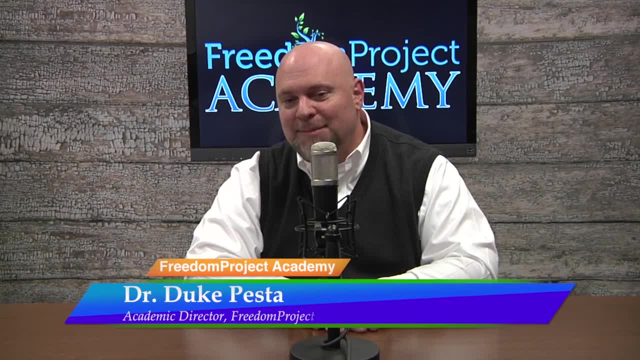 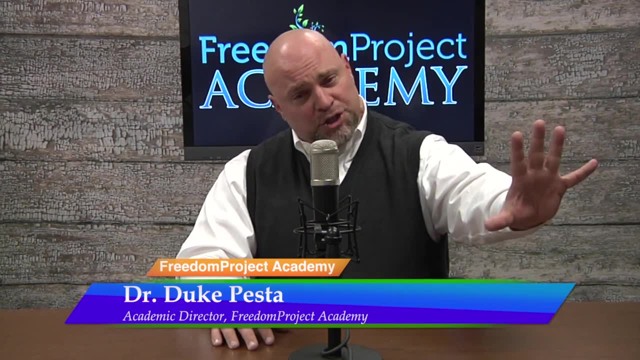 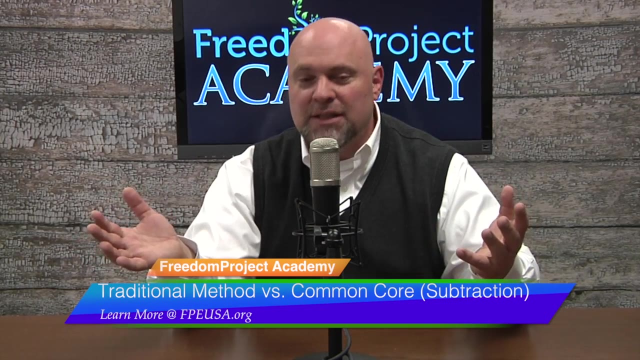 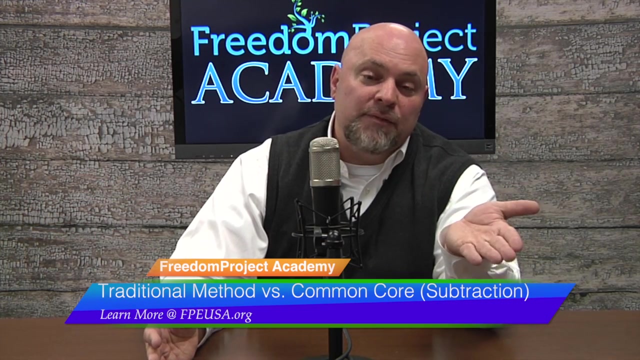 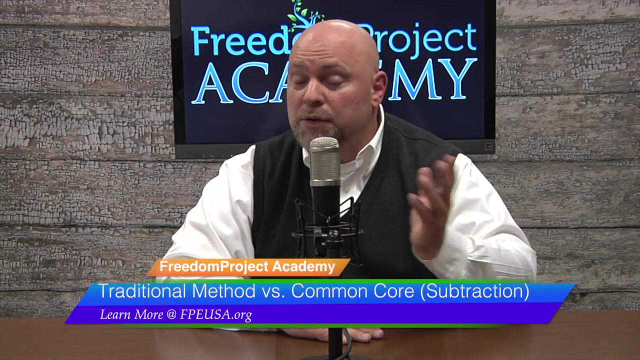 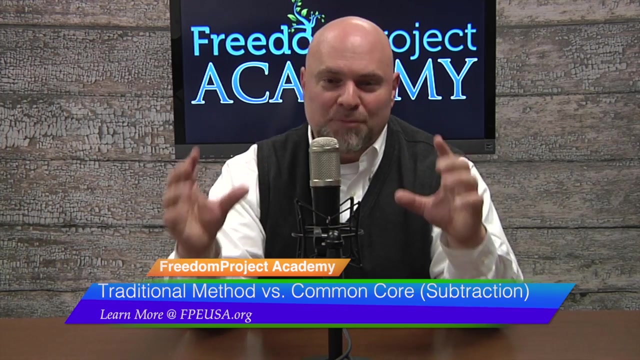 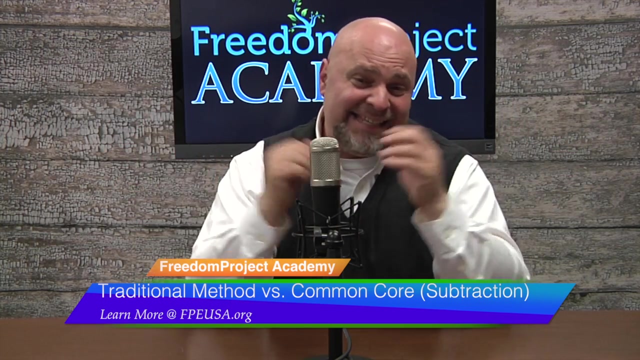 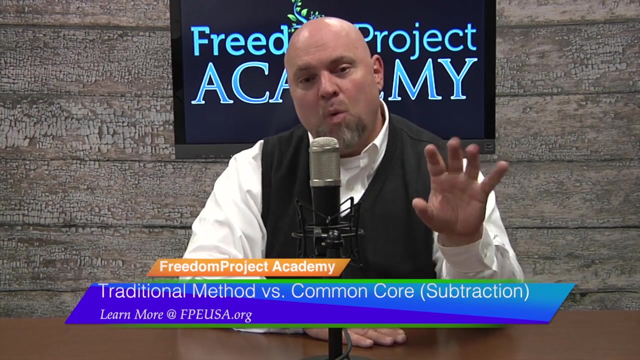 Hi everybody, Dr. Duke, Academic Director of Freedom Project Academy coming at you with yet another of our Common Core Math comparisons. We have a number of them on our website where we compare traditional math to the Common Core Math. We show you at various grade levels the insanity, the obfuscation, the mindlessly obtuse way that Common Core Math goes about its business and this simple elegance of traditional math which you can no longer do in Common Core Math classrooms. Today we have an interesting example coming from Mary Black who's done our whole series. Mary Black is our Curriculum Director and she's looking at something as simple as subtraction. Now you wouldn't think subtracting one number from another would be complicated, would require multiple steps, would require all sorts of arcane examples and needlessly extended work, but that's exactly what happens with Common Core. So take a look as Mary Black walks you through traditional subtraction and shows you what they're doing to your kids with Common Core. 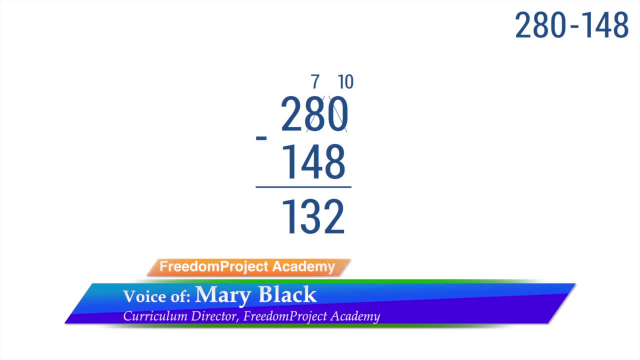 Let's solve a subtraction problem using the traditional right to left method. The problem 280 subtract 148 is shown. Because 8 can't be subtracted from 0, we borrow a 10 from 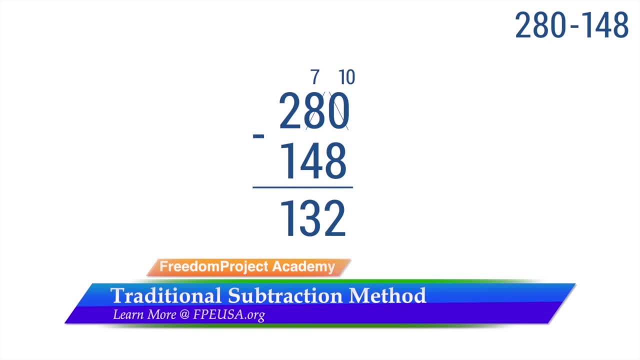 the 8 in 280, leaving us with 7, and we add 10 ones to the 0. Going from right to left we subtract 8 from 10, 4 from 7, and 1 from 2 to get the difference between 8 and 10. We subtract 8 from 10, 4 from 10, and we add 10 from 10, and we subtract 3 from 10. We subtract 9 from 10, 4 from 10, and we subtract 1 from 10, and we subtract 5 from 10, and we subtract 1 from 10, and we subtract 5 from 10. 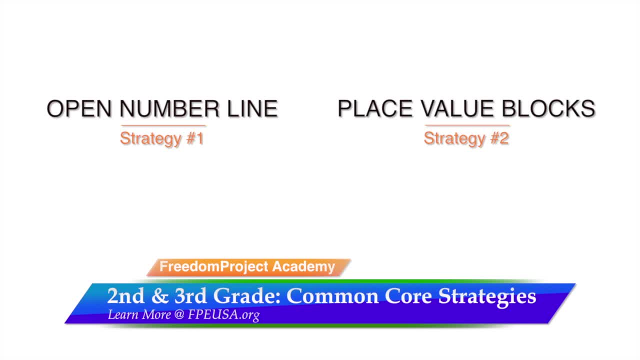 Common Core teaches arithmetic by presenting multiple strategies. The first two we'll discuss 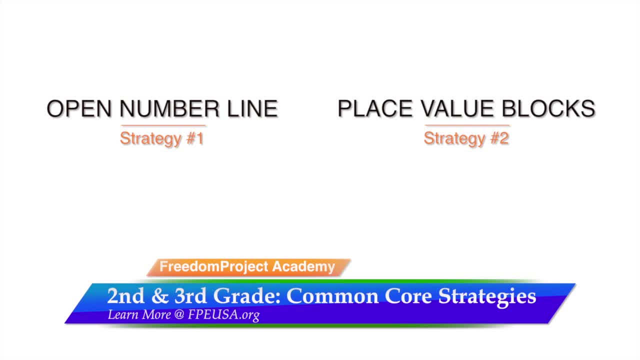 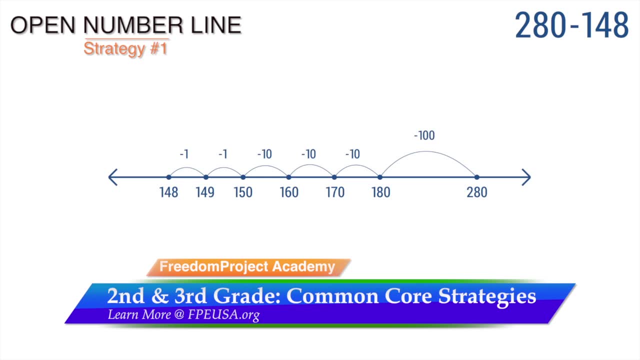 are intended for second and third grades. The first is the open number line. This does not require knowledge of facts or the use of borrowing. We simply count down the number line and add up our leaps to solve the problem. The second early elementary strategy is to is place value blocks. Again, we do not need to know subtraction facts. We begin by drawing two hundreds and eight tens. We simply cross out a ten 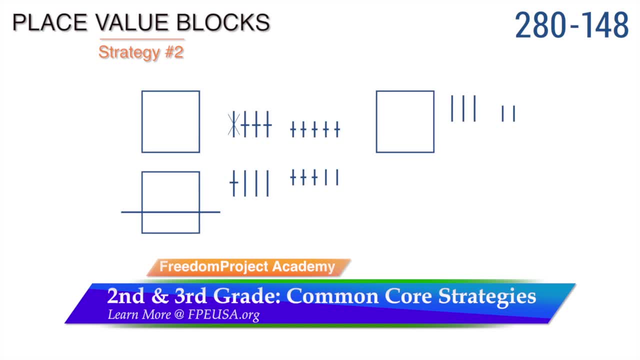 to give us ten ones so we can mark through 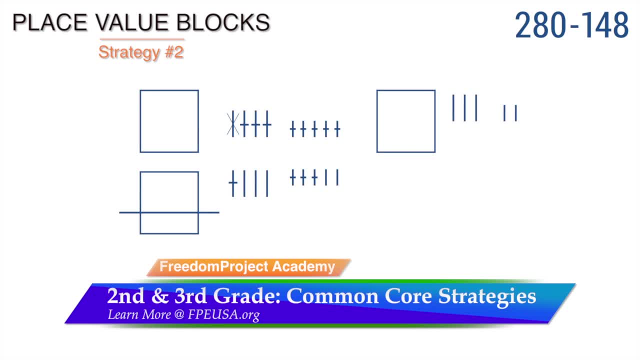 eight ones, four tens, and one hundred. 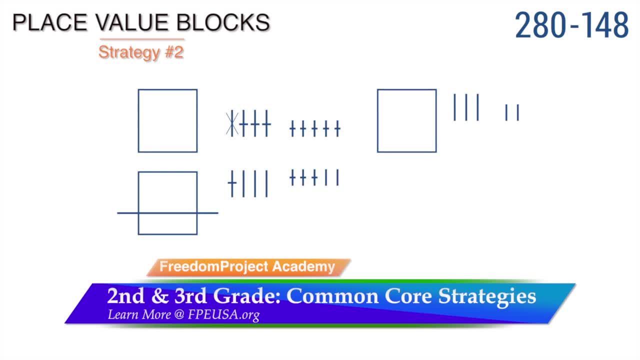 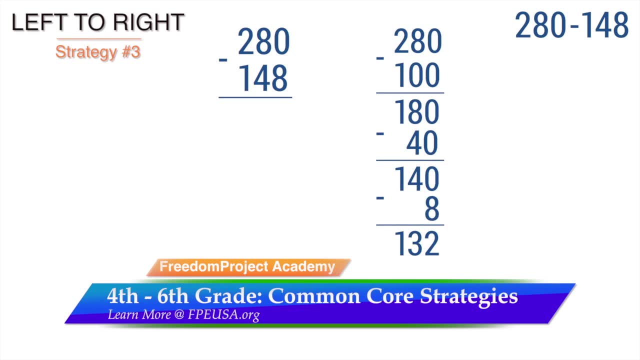 You see what is left on the right hand side of the screen. Now let's look at some upper elementary strategies. The left to right or mental math strategy is not only simplified and watered down, but it trains the children to subtract from left to right, which leaves students confused and unable to use the traditional right to left method. 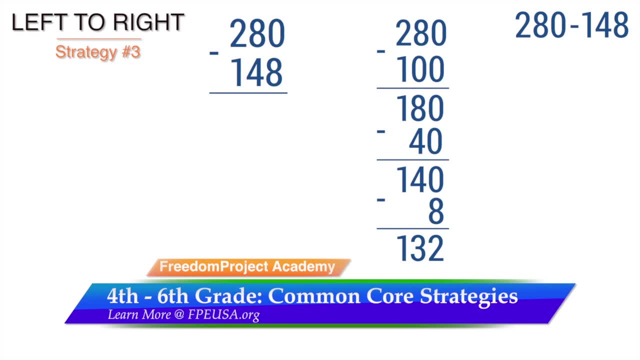 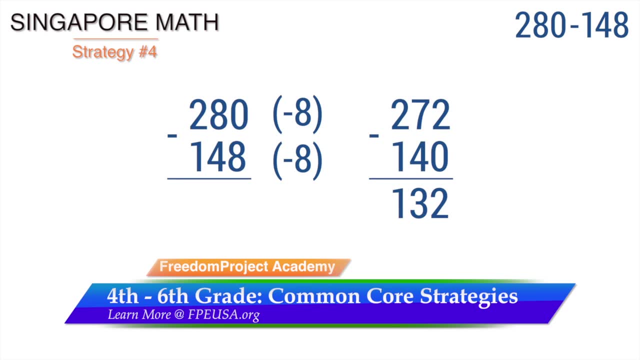 The students reach higher levels of math, unable to subtract without resorting to one of these strategies. The Singapore math strategy. This strategy avoids borrowing by subtracting eight from two hundred and eighty and one hundred and forty-eight. I am not certain how one can say that no borrowing took place when eight was subtracted from two hundred and eighty. 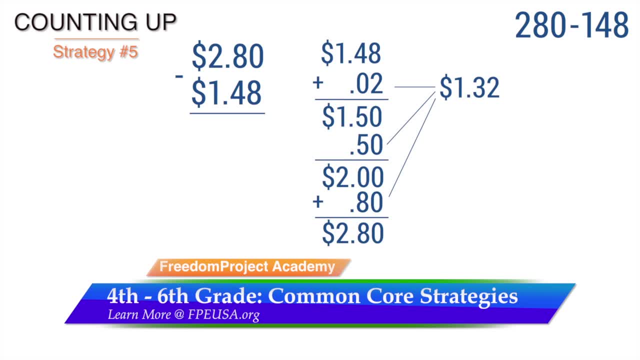 Counting up or giving change. In this method, two hundred eighty is changed to two dollars and eighty cents and a hundred and forty-eight is changed to a dollar and forty-eight cents. And increments of money are added to a dollar forty-eight to reach two dollars and eighty cents. 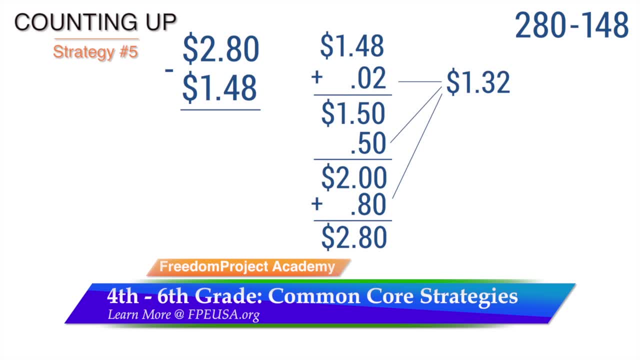 This is not even the proper method to give change. 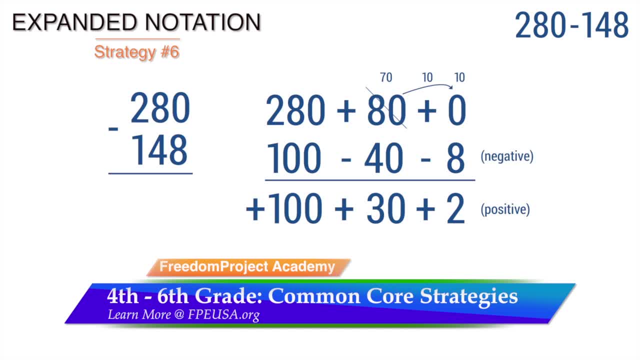 Expanded notation. This is the most popular strategy. 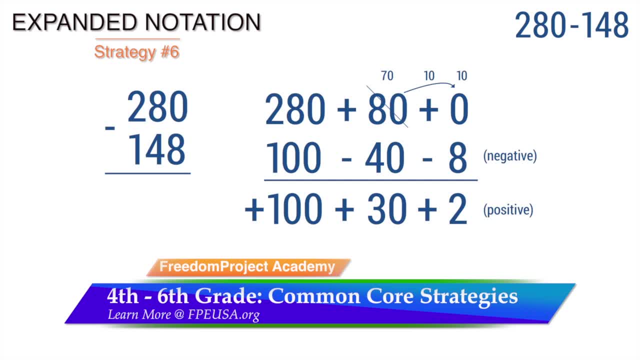 Notice the use of the terms negative and positive numbers before the student is capable of subtracting in the traditional and efficient manner. 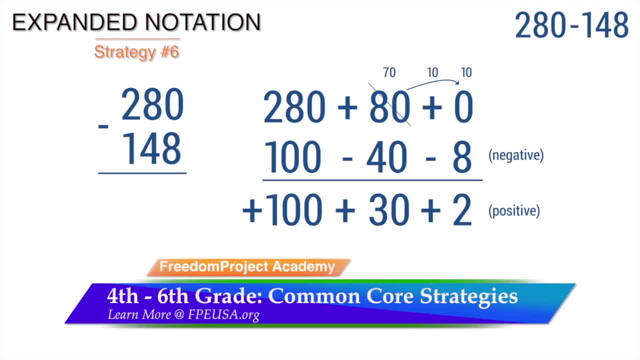 How does this affect students? At higher levels of math. 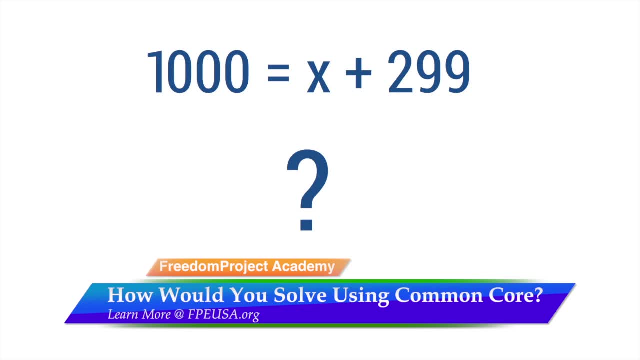 One thousand equals x plus two hundred ninety-nine is an example of an equation pre-algebra or algebra one students would be asked to solve. 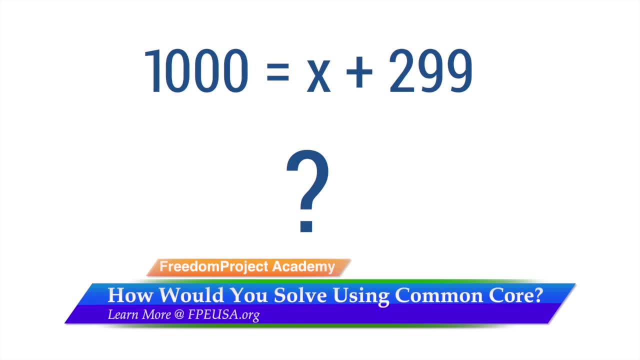 To solve for x, one must subtract two hundred ninety-nine from both sides of the equation. It is likely that the students will have to resort to using one of these strategies we have discussed or a calculator if he or she was not lucky enough to learn the traditional right-to-left method of subtraction.